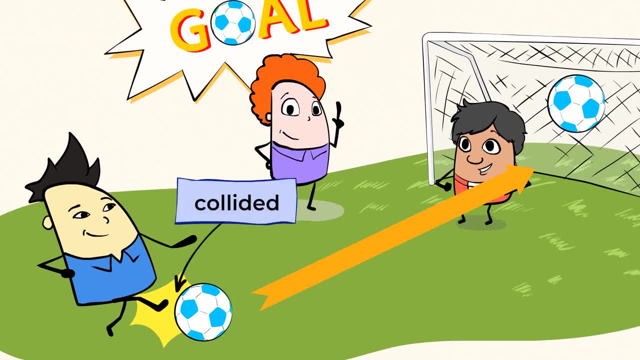 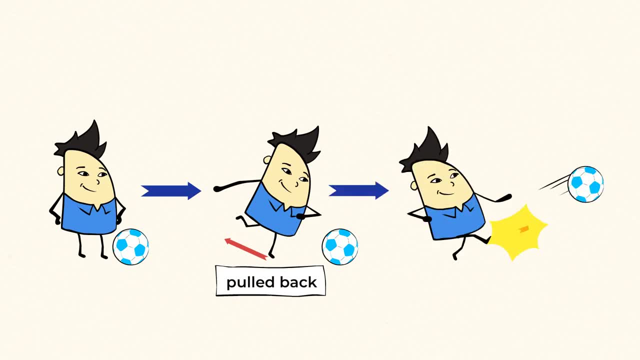 Wow, When Chen's foot collided with the ball, it put it in motion, and that was quite a kick. Chen pulled his leg way back and struck the soccer ball with a lot of force and speed. Well, it looks like a lot of energy was transferred from his leg to the ball. 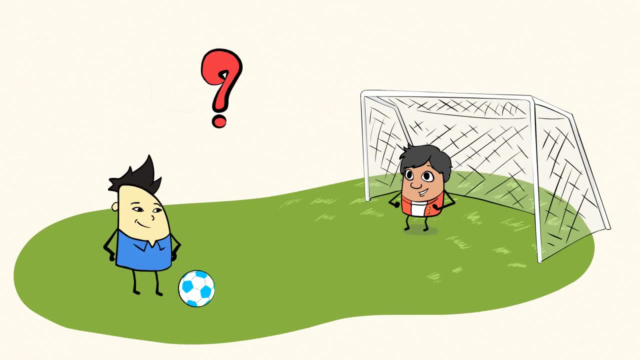 No wonder he scored. Now let's see what happens if Chen kicks the ball more softly. Okay, well, that ball did not go very far. So when Chen moves his leg slowly and does not kick the ball with much force, 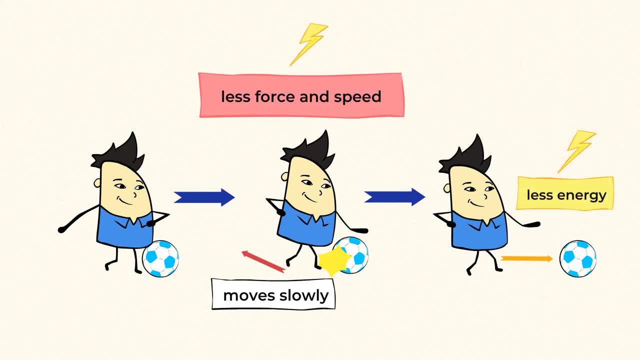 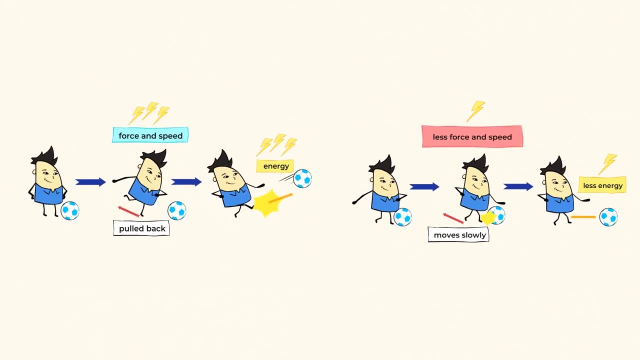 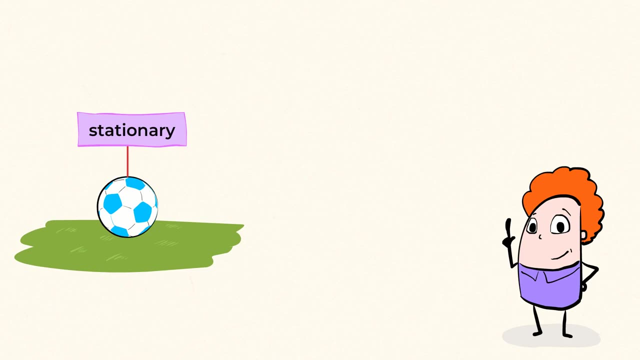 well, there's less energy going from his leg to the ball And even though they are still colliding, the ball travels slower and doesn't travel nearly as far. Now this example is a little different from the baseball, because the soccer ball is stationary, or still when it collides with the foot. 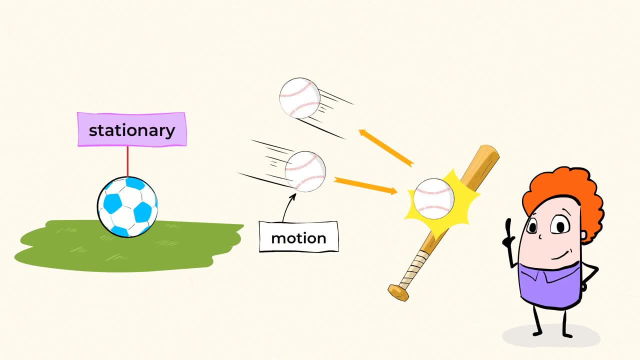 The baseball is already in motion and the collision with the bat completely changes the direction that the ball is going. The baseball is already in motion and the collision with the bat completely changes the direction that the ball is going. The baseball is already in motion and the collision with the bat completely changes the direction that the ball is going. 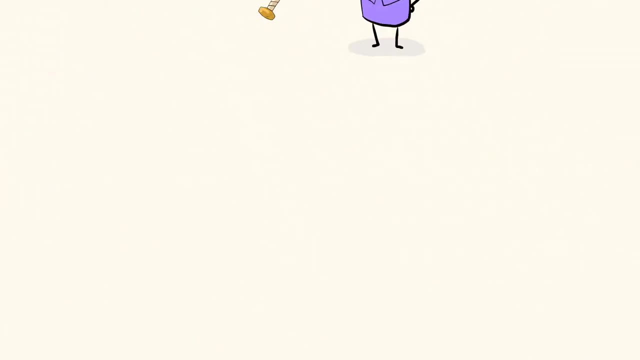 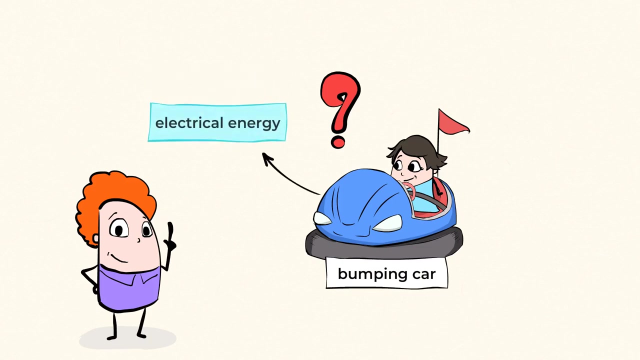 Huh, that's an interesting idea. Let's explore it further. Have you ever ridden in bumper cars? Well, if you have, you know what a wild ride it can be. Bumper cars use electrical energy to move around, Oh look. 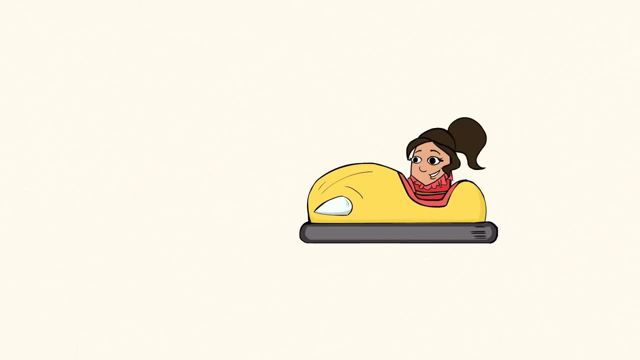 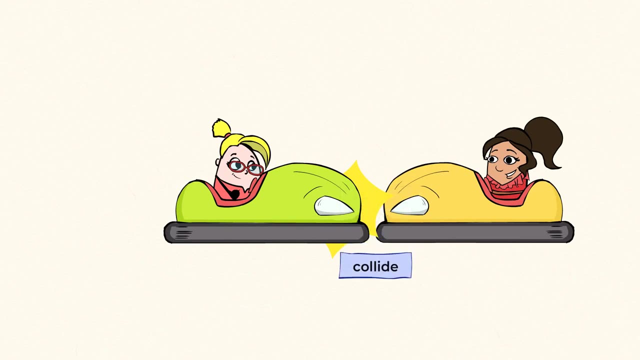 There's Isabella riding around in her yellow bumper car. Oh, watch out. Another car is headed her direction and BOOM, The two cars collide. Now the car that is going faster has more energy, and that energy is transferred to the other, slower-moving car. 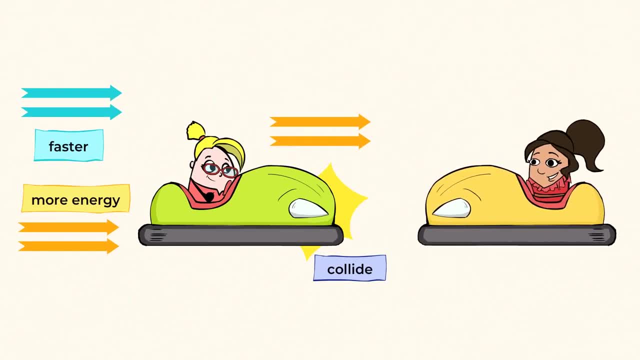 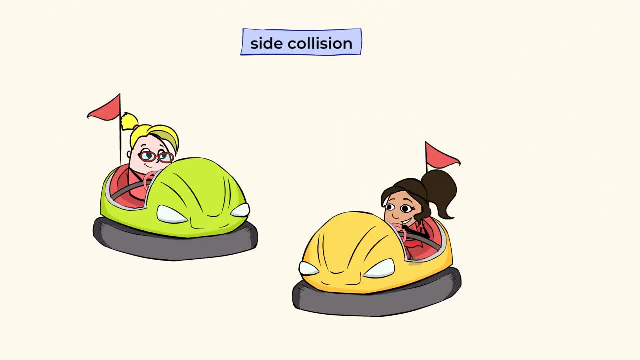 If they crash head-on, the faster-moving car will push the other car backward in the opposite direction it was traveling. But what happens if there's a collision on the side of the car? Well, with a side collision, energy is transferred. 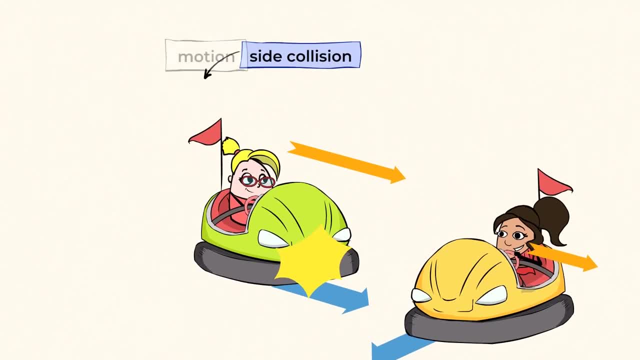 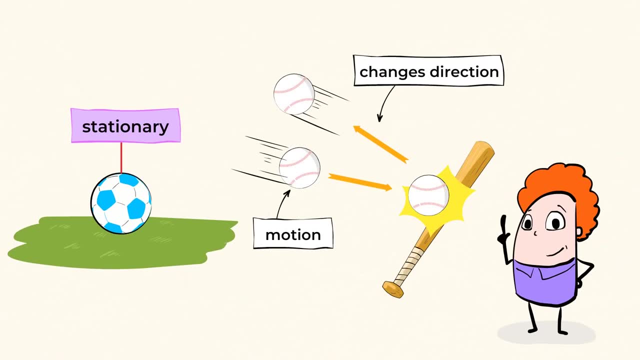 and the other car is pushed sideways. So a collision does not just put things in motion, it can actually change the direction that objects are traveling in. And just like the baseball and the bat, both are moving and one causes the other to change directions.